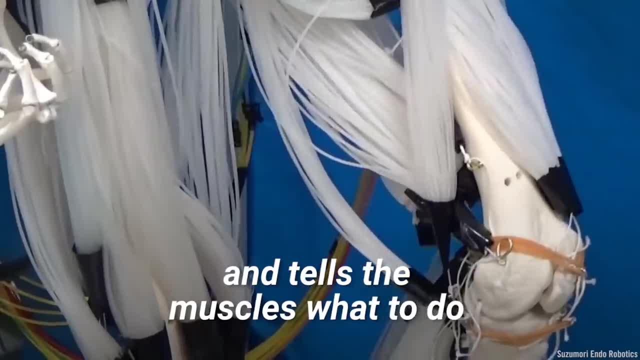 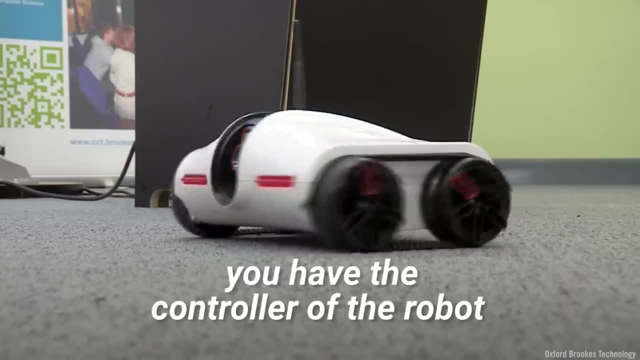 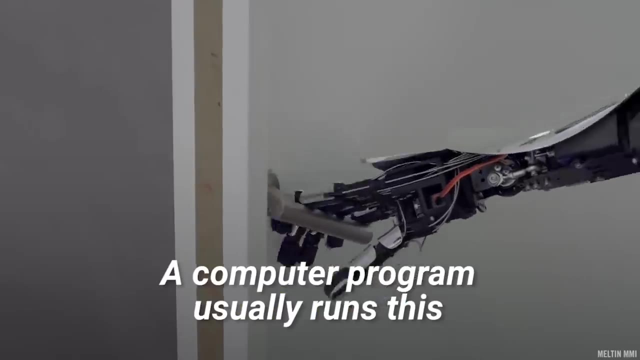 a brain that processes sensory information and tells the muscles what to do. Many types of robots also include these systems. 1. You have the controller of the robot, which could also be called the brain of the robot. A computer program usually runs this and it gives the robot detailed commands to follow. 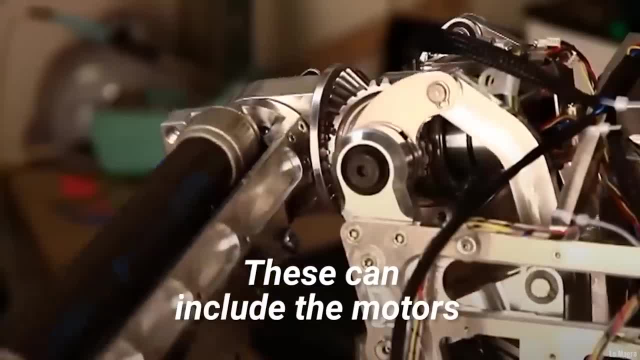 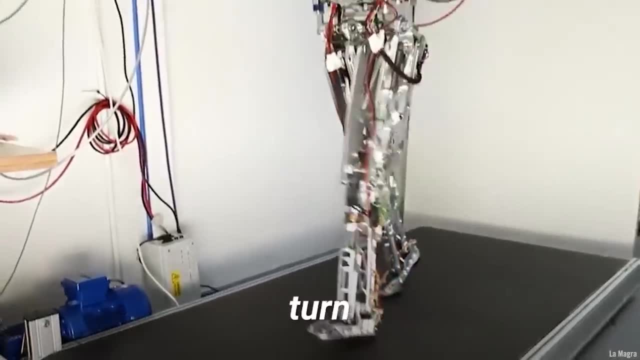 2. You have mechanical parts. These can include the motors, pistons, grippers, wheels and gears- and help the robot move: grab, turn and lift. They are usually powered by air, water or electricity. 3. 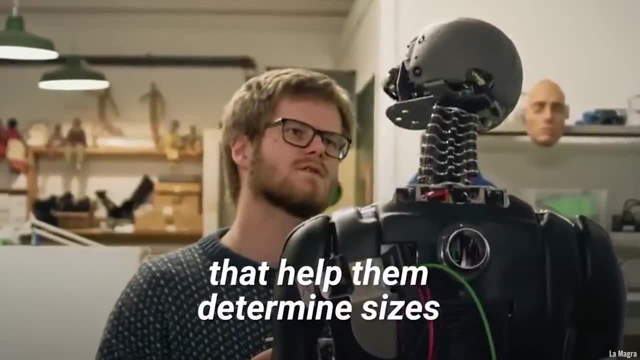 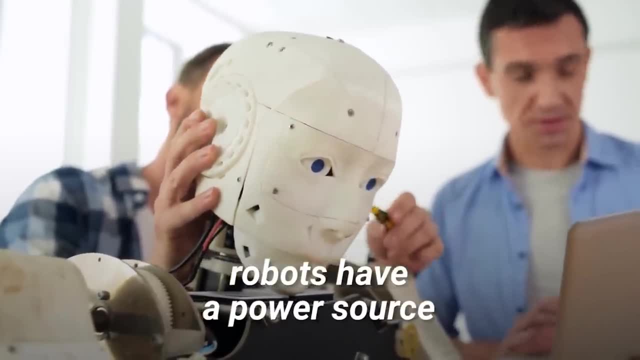 Robots also have sensors that help the robot move, grab, turn and lift. They are usually powered by air, water or electricity. 4. Robots have a power source. All of these components work together to control how a robot operates. 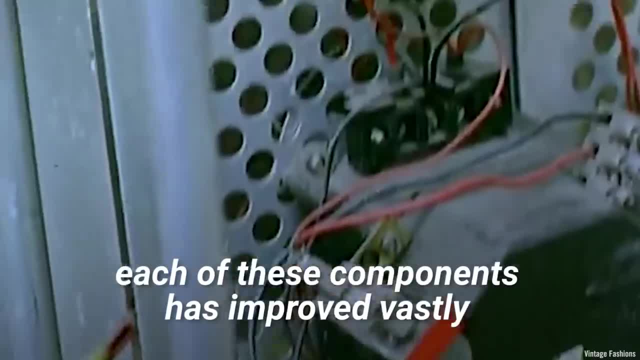 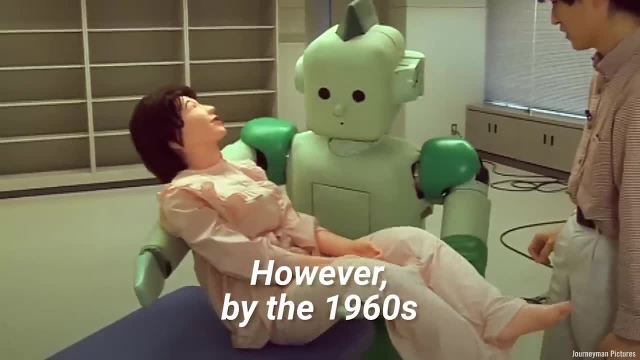 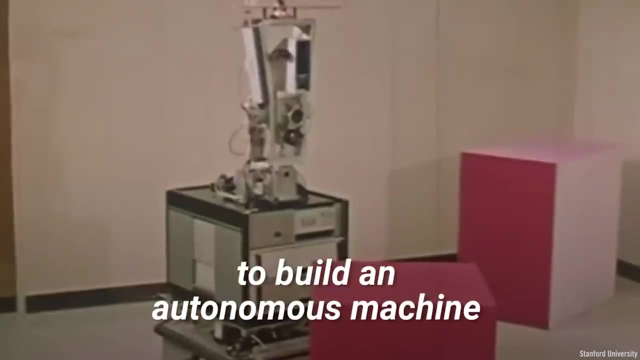 Throughout the history of robotics, each of these components has improved vastly. Robots have been a longstanding trope in science fiction. However, by the 1960s they were actually becoming a reality. 5. The first real effort to build an autonomous machine that could move, reason and act. 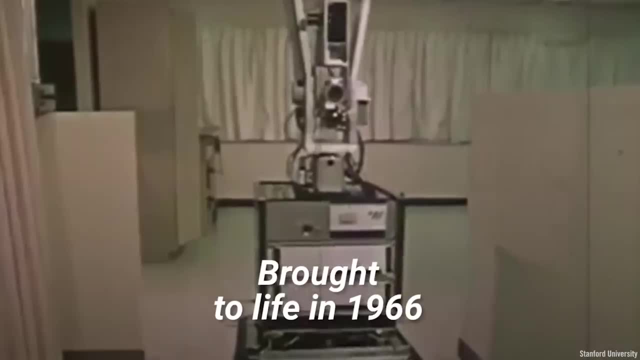 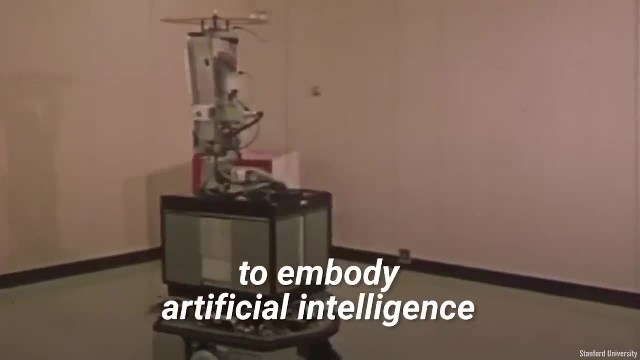 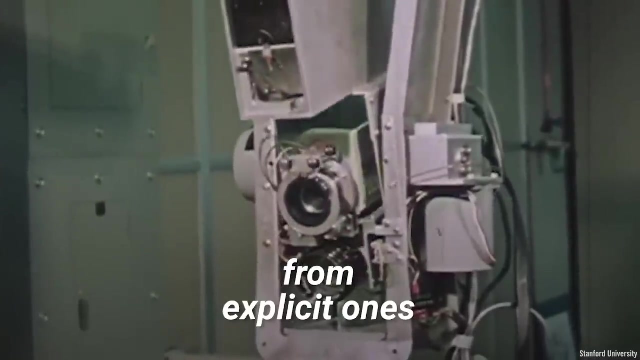 in its environment was the robot Shakey. Brought to life in 1966,, Shakey is considered to be the world's first robot to embody artificial intelligence. Shakey could perceive its surroundings logically, deduce implicit facts from explicit ones, make a plan to achieve a goal, monitor the execution of a plan in the real world, and 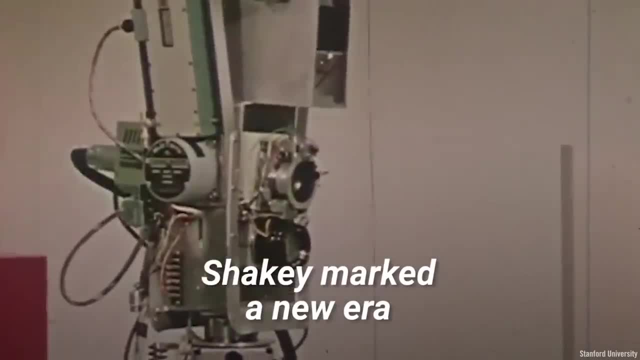 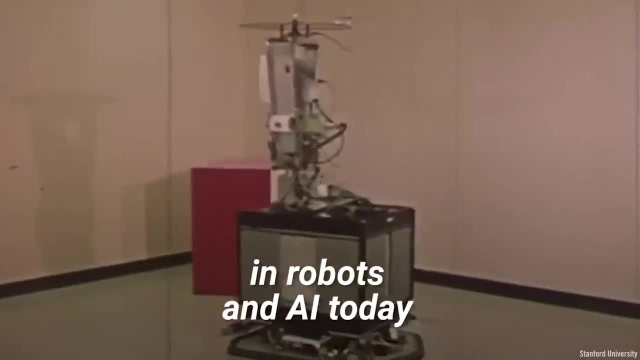 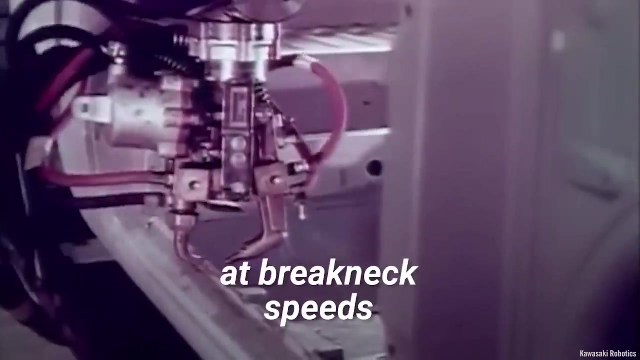 even correct its own errors. Shakey marked a new era in the age of robotics and computer science. Some of the algorithms used in robots and AI today have directly descended from Shakey. The area of robotics has evolved at breakneck speeds. Companies like Boston Dynamics are 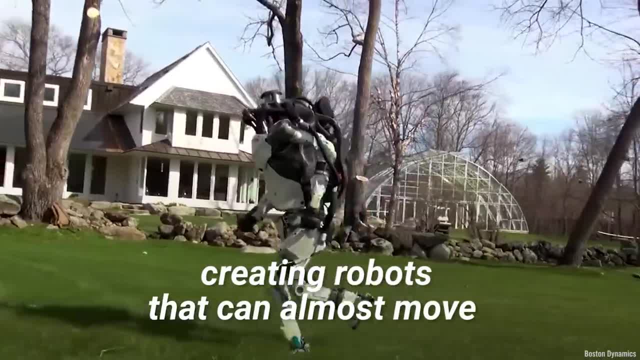 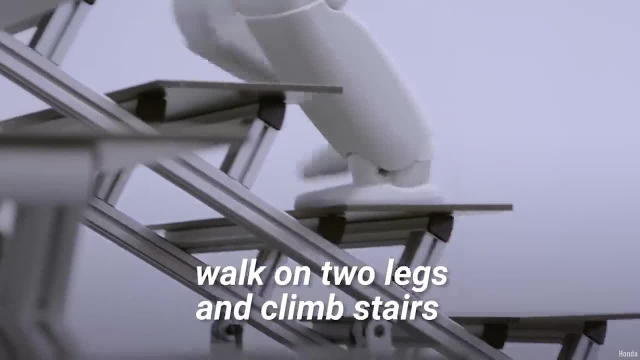 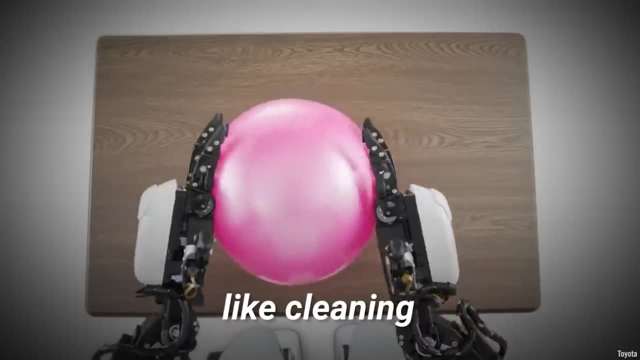 leading the charge, creating robots that can almost move as well as you. Honda's Asimo can learn independently, walk on two legs and drive 4.. Toyota's THR3 humanoid robot has been designed to fill a wide range of roles like cleaning.